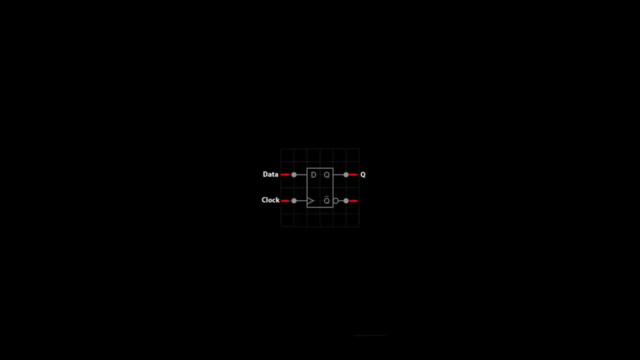 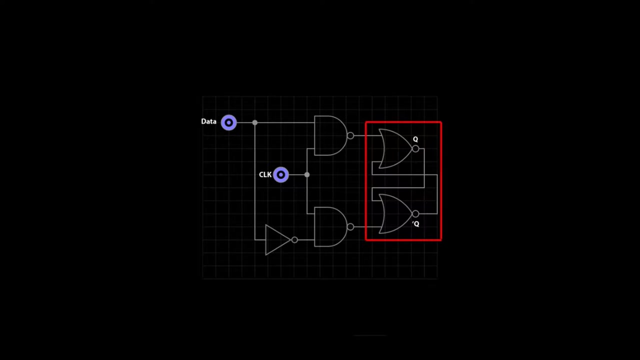 The outputs are labelled Q and Q0.. Q0 is the inverse of Q. This is the logic diagram for a D flip-flop. Notice that the NOR flip-flop is used in the circuit with other logic gates added. This helps to prevent the do not use condition found in the basic norm. 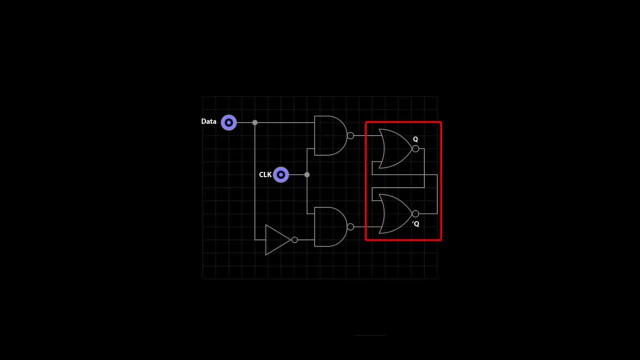 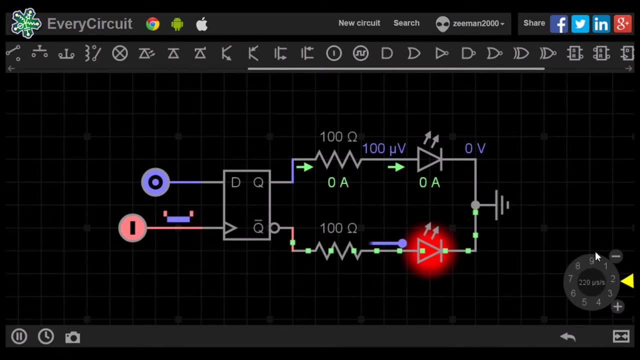 The truth table for this circuit is as follows: When the clock pulse is at zero and D is at zero, there is no change on Q or N running on the clock input. this can be seen clearer by increasing the simulation speed. when d has a zero input, then q naught remains high. when we change the d input to one, q then becomes. 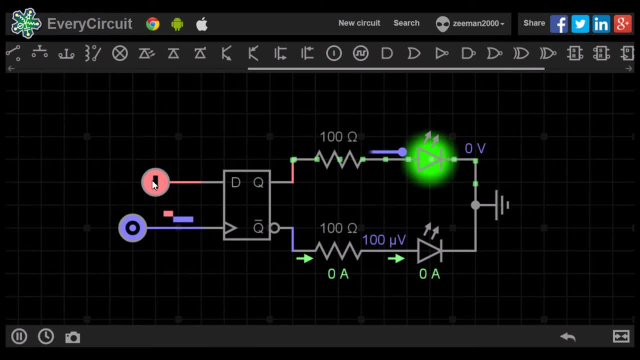 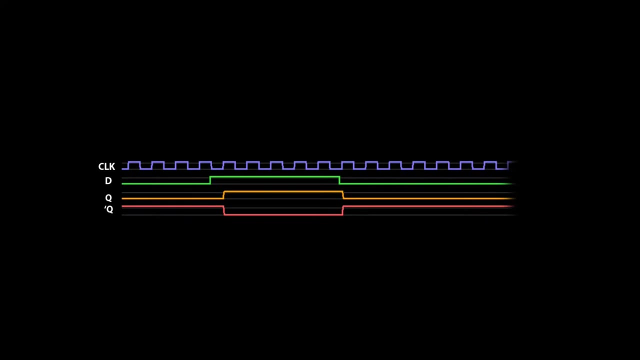 high. when we change d back to zero, q goes back to low and q naught becomes high. let's examine the waveform output to look at what the input and output signals are doing. here we can see the waveforms produced when we tested the d flip-flop. 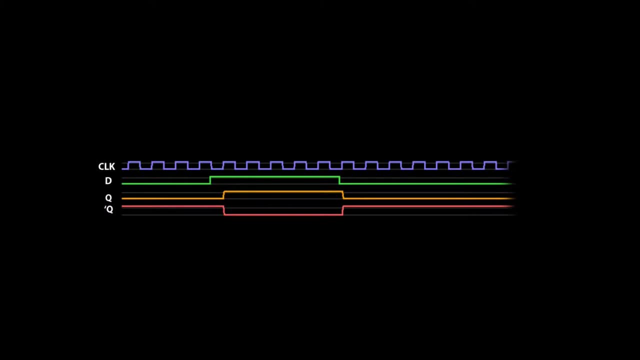 this is the output for clock: d, q and q naught. when we started the simulation, the clock pulse was rising and falling constantly, providing a zero one input. d was at zero and q was also at zero and q naught at one notice that when d is then set to one, q and q naught do not change until the next. 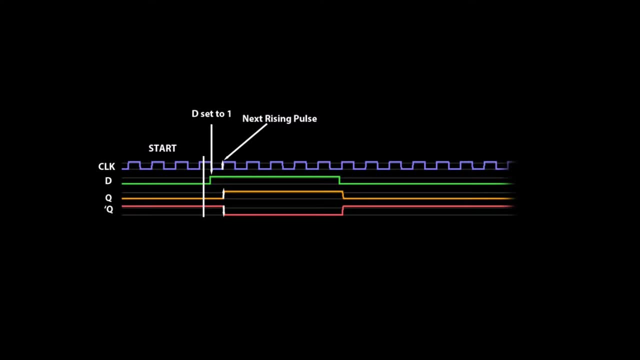 right rising clock pulse. when we change d back to zero, q goes to zero and q naught to one again. this happens on the next rising clock pulse. let's go back to the simulator to examine some practical applications for the d flip-flop so we can understand the circuit better. 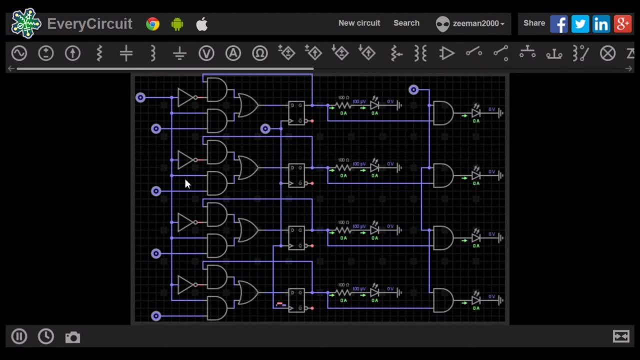 this circuit is a model of the d-flip-flop, which is a two-dimensional circuit of a 4-bit data register. The purpose of this circuit is for a binary input to be placed into the circuit, which is then stored in memory, then output to a data bus. 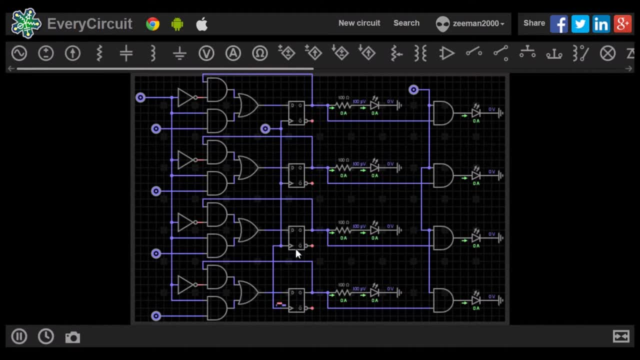 This circuit has four D flip-flops which are controlled by the same clock pulse. There are some logic gates which connect to the D input. They consist of an OR gate, two AND gates and a NOT gate. Each of the flip-flops have these logic gates at the D inputs. 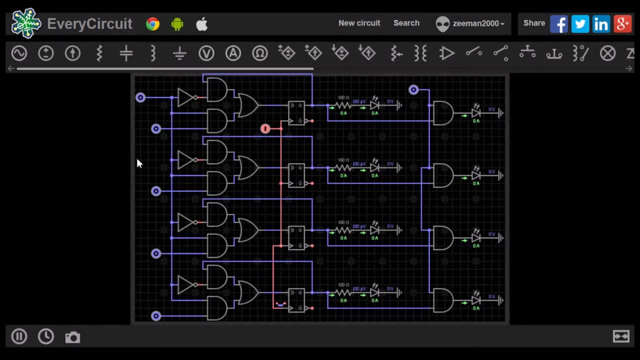 The logic gates in this configuration are also known as a multiplexer. Each of the multiplexers are tied together with a D input, The top input switch. This switch is called the enable switch. It controls when the data is written to memory. 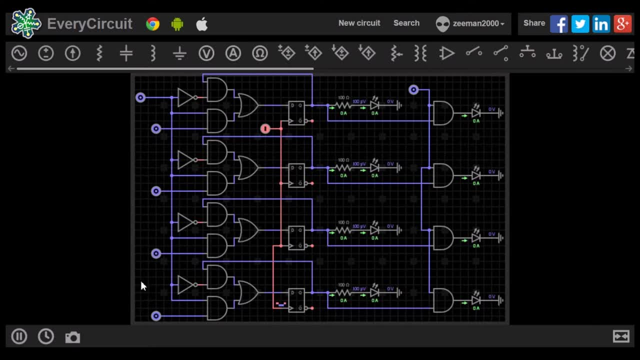 The lower input switches are data switches. They are binary inputs which connect into each multiplexer and represent the binary value of 1,, 2,, 4, and 8.. The LEDs at the Q output of each flip-flop will light when a 1 is written to memory and will stay off when a 0 is written to memory. 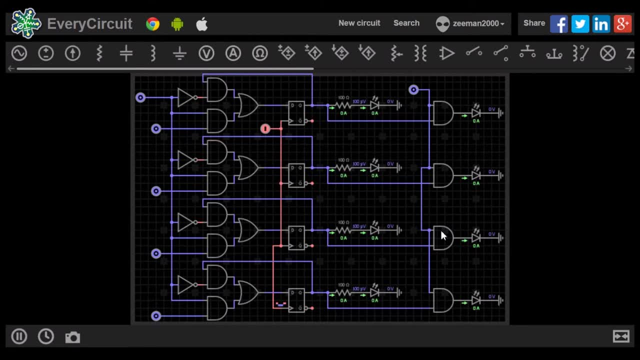 The AND gates furthest to the right have one of their inputs connected to Q. The other input of the AND gates are all tied together and are then connected to an input switch. This part of the circuit is to control when the data in memory is output to another external circuit. 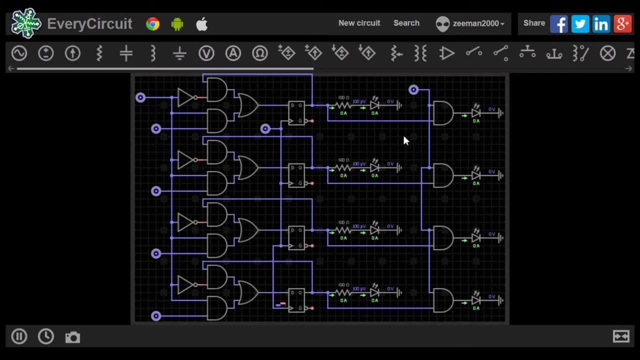 To use the circuit, we first need to input a binary value. so we will enter 1010.. To write the data to memory, we need to turn the enable switch on. To write the data to memory, we need to turn the enable switch on. 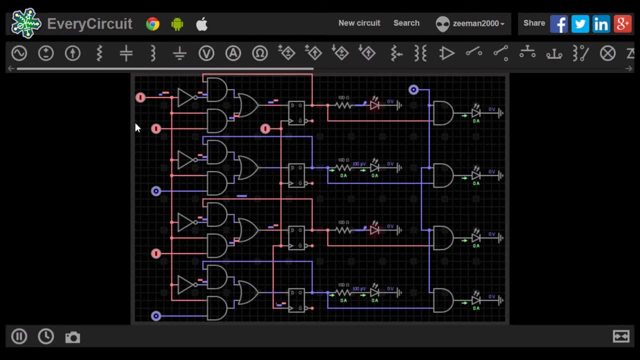 To write the data to memory, we need to turn the enable switch on. This data is now written to memory. Before we can write another binary input to memory, we need to set enable back to 0.. Notice, our input of 1010 is still stored. 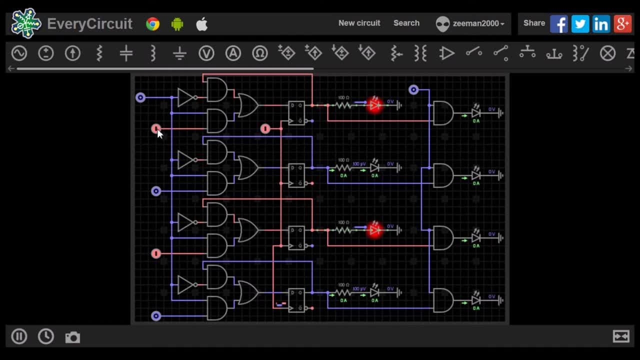 We can now input a new value of 010.. We can now input a new value of 010.. We can now input a new value of 010.. When we set enable to 1, the new value is written to memory. When we set enable back to 0,, this holds the value. 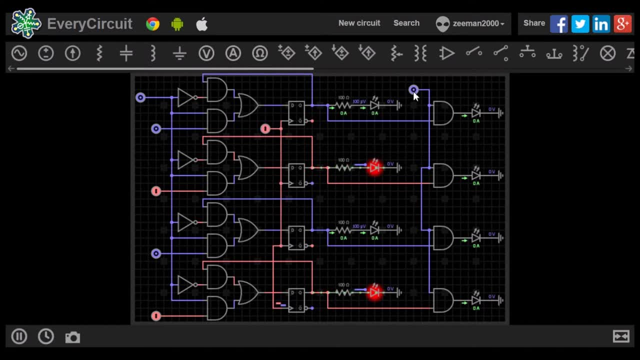 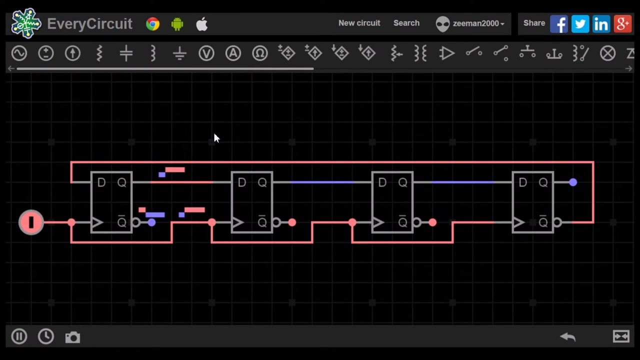 We can now turn the output switch on to simulate outputting the data from memory to an external circuit. Let's now examine another practical application. we can build with D flip-flops With this circuit. we have used the D flip-flops to create a ring counter. 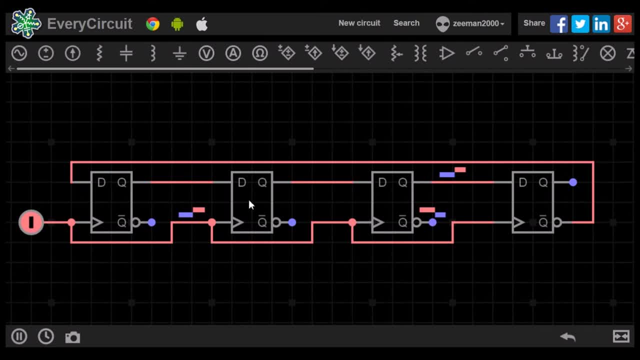 We have four D flip-flops side by side. The clock speed is 10 milliseconds and simulation speed is 19 points. We have a logic train input which is linked to the clock inputs of each flip-flop. The Q output of each flip-flop is connected to the D input. 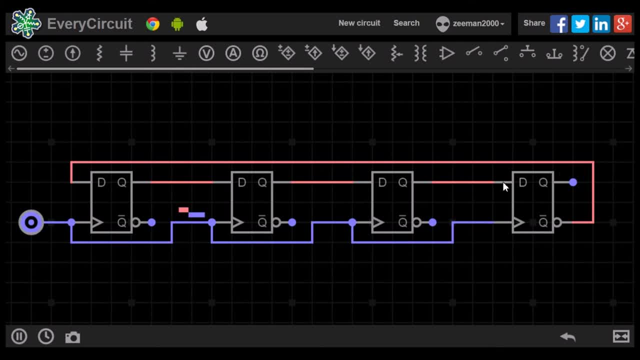 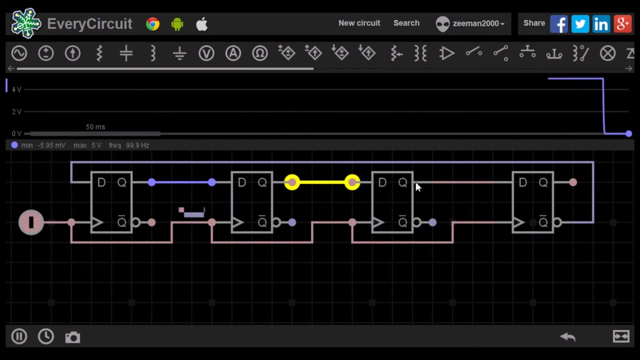 The Q0 output of the last flip-flop connects back to the D input of the first. Let's highlight the Q0 output of the last flip-flop. Let's highlight the Q0 output of the last flip-flop. Let's highlight the Q0 output of each flip-flop to examine what is happening on the waveform viewer. 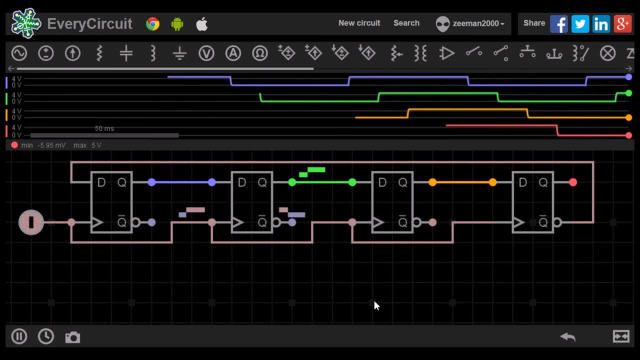 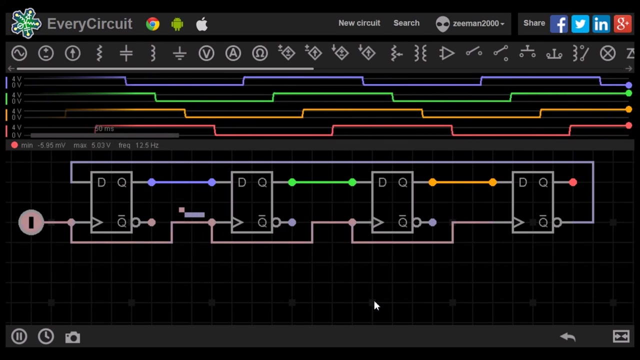 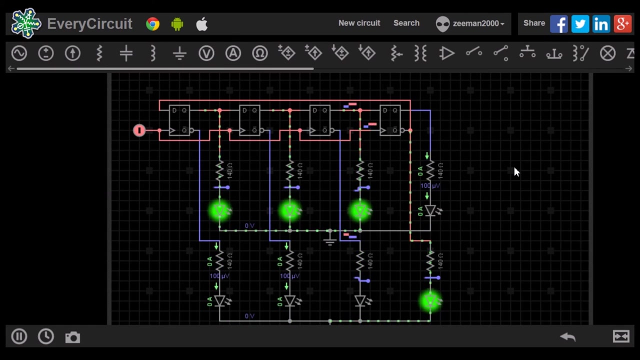 As we can see, Q on the first flip-flop goes high, then the second, then the third, then the fourth. One goes high after the other in succession. One goes low after the other in succession. We can connect LEDs to the Q and Q0 outputs to examine the signals outputs. 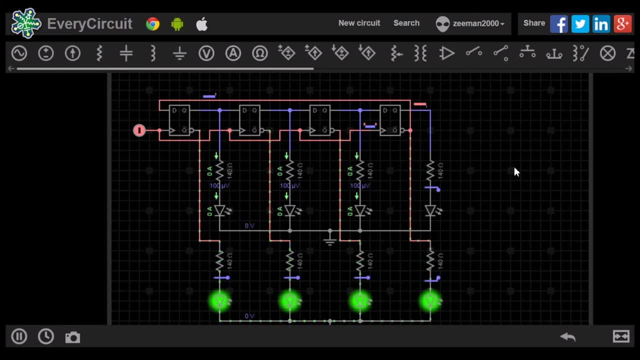 As we can see, the LEDs light up in a 1-2-3-4 succession, then turn off in 1-2-3-4 succession, Then turn off in 1-2-3-4 succession. The Q0 output does the inverse. 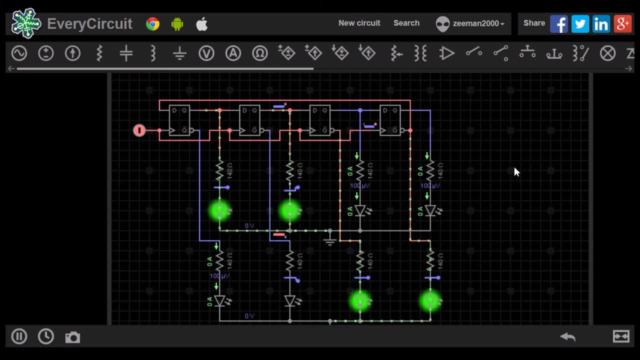 This type of circuit would be used as a type of shift register in logic applications. This type of circuit would be used as a type of shift register in logic applications. The D flip-flop has applications in computer memory- binary counters and shifters, and they are common in computer circuits.